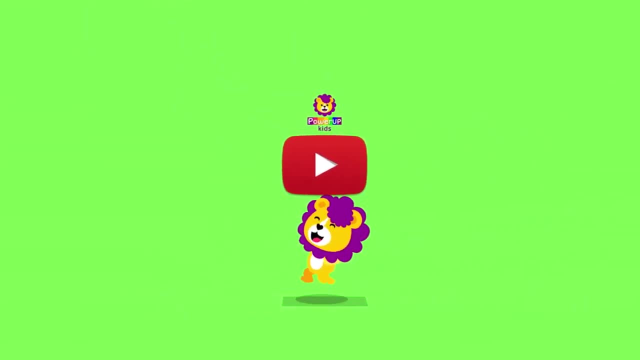 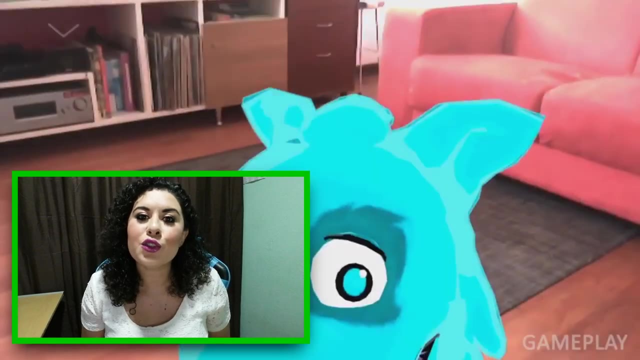 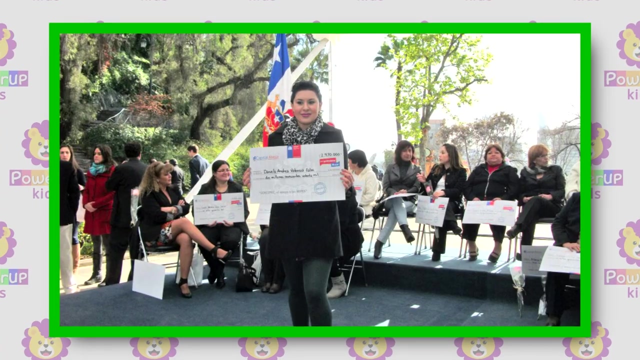 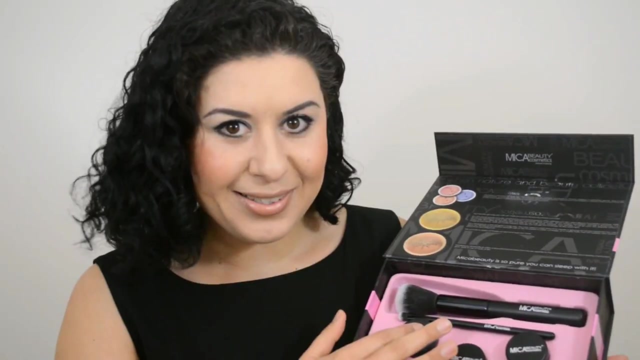 That was how Power Up Kids was born. Power Up Kids- Power Up Kids- is one of the most experienced video game audio experts and cartoon musician in Chile, with more than 100 video games on his portfolio. Myself have been an entrepreneur and artist in the audiovisual and video game industry and, at the same time, have been working in sales and marketing. 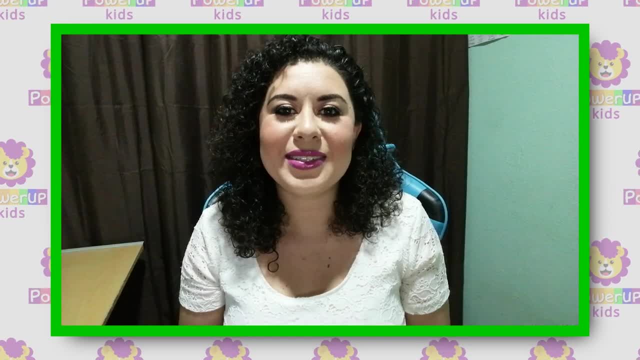 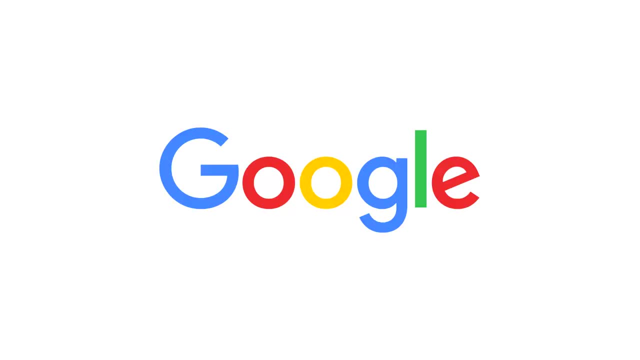 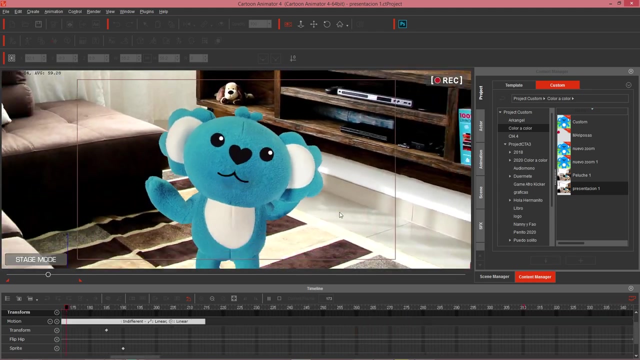 We both have been working together since 2007 in projects for companies as Nintendo Cartoon Network and the NintendoIC, as Nintendo Cartoon Network, Nickelodeon and Google Cartoon Animator 4 made possible our project as it is a fantastic software easy to use. 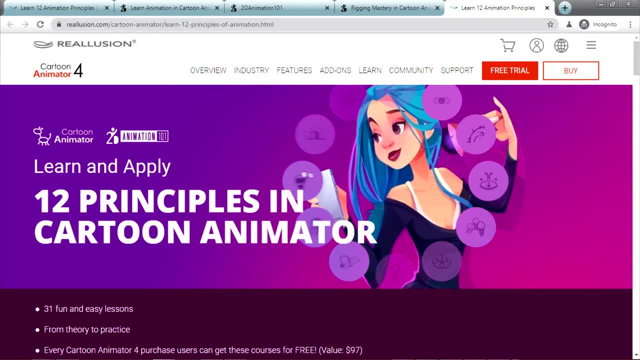 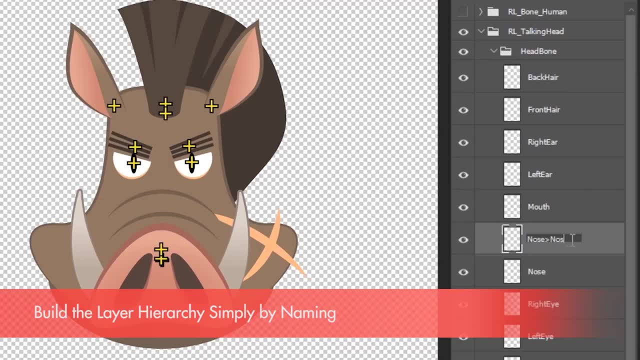 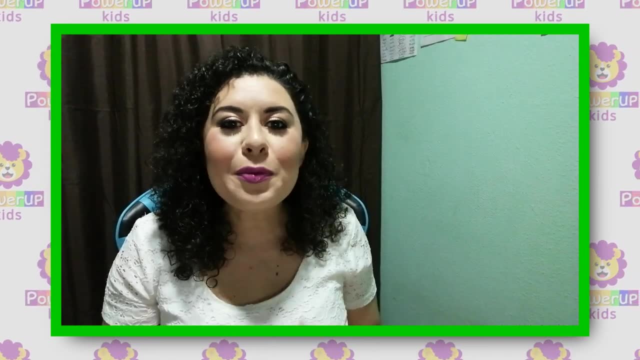 with a friendly interface and a lot of online courses, tutorials and webinars that help us a lot to learn how to use it, plus a lot of tricks and techniques to power up our animation. Another important fact about Cartoon Animator 4 are the pre-made animations that can be. 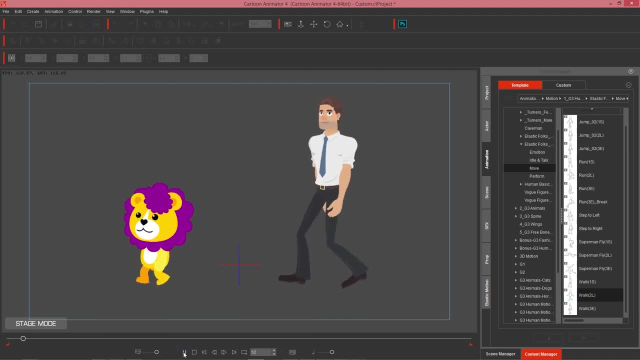 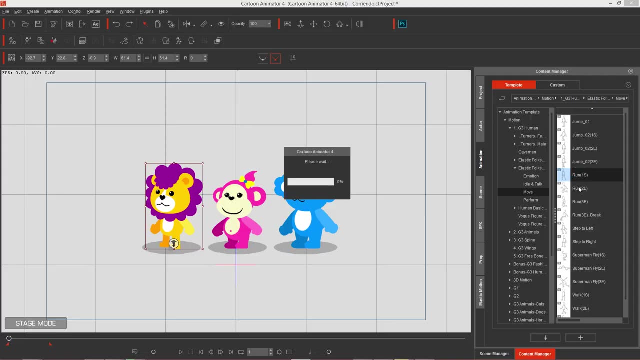 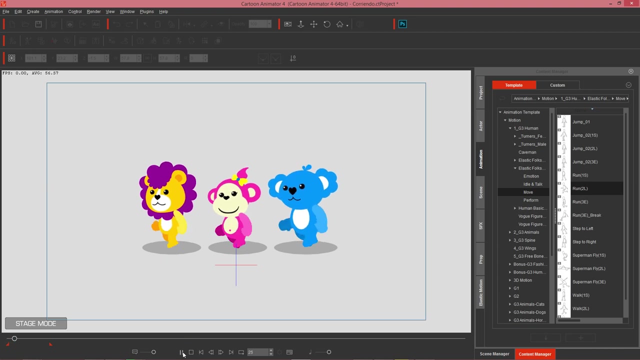 easily retargeted to different characters. As Power Up Kids has several characters, it would be time-consuming to animate them one by one. Instead, with the pre-made motions, we can apply them all at the same time. Moreover, the props included in the software saved us a lot of time. 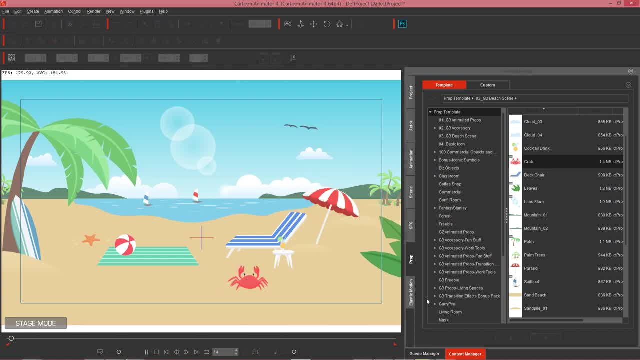 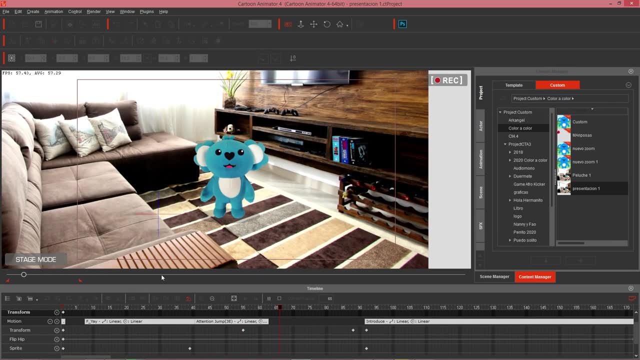 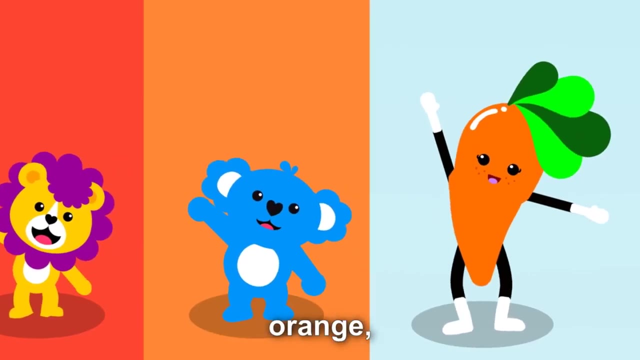 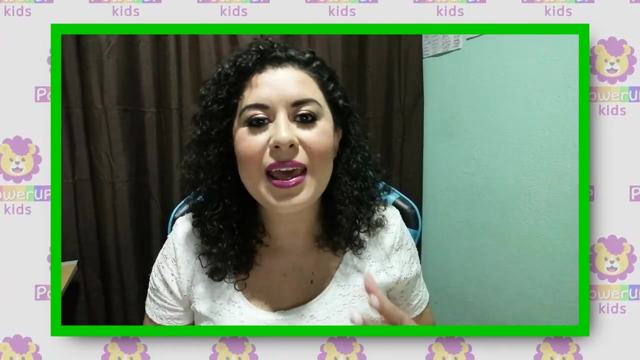 Any of our video clips could have taken over two months of work with any other animation software, but with Cartoon Animator 4 we made it in less than two weeks with no experience at all in animation. In addition, if all the pre-made motions and props included in the software are not enough, 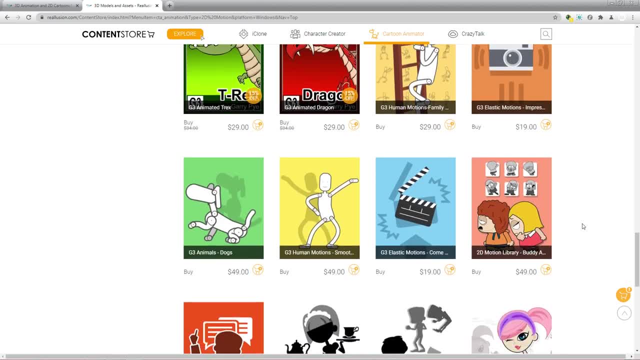 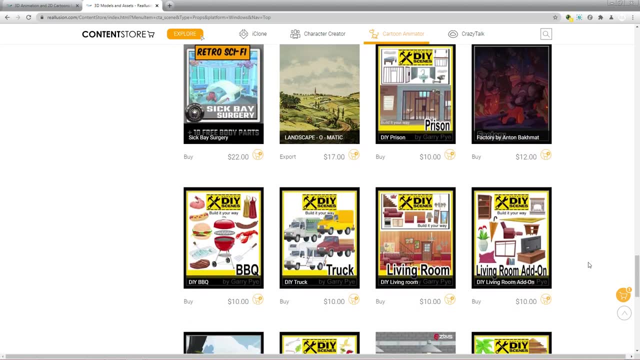 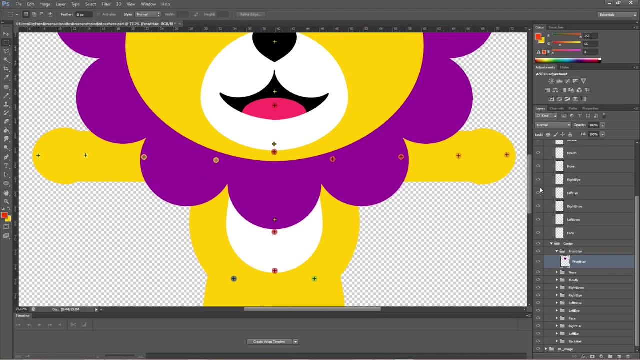 we can always count on the real work. The animation software is also very useful for us Content Store, where you can get tons of pre-made animations and props to keep saving time. The results we got are amazing and, as we both have experience working with Photoshop, it was super easy for us to create characters using the